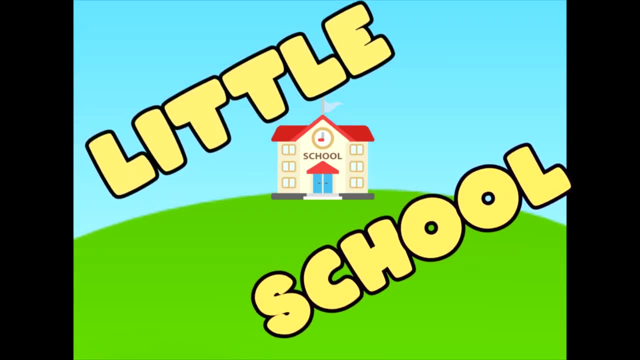 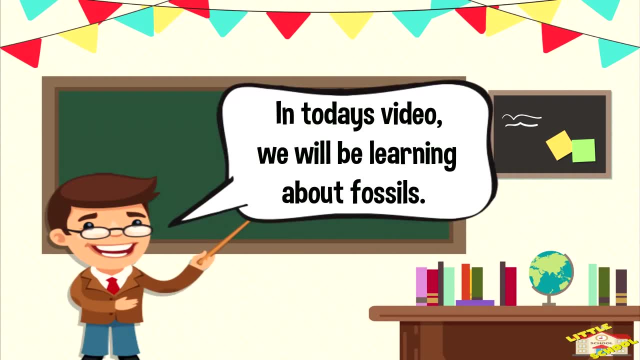 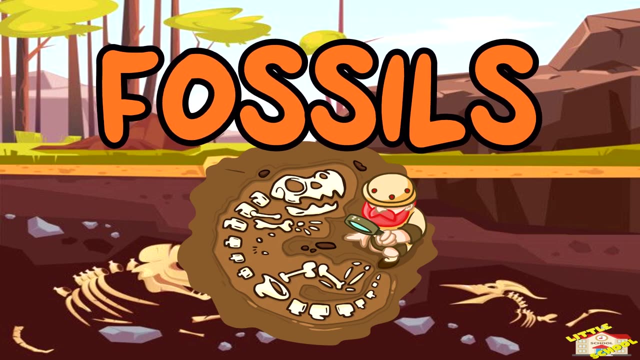 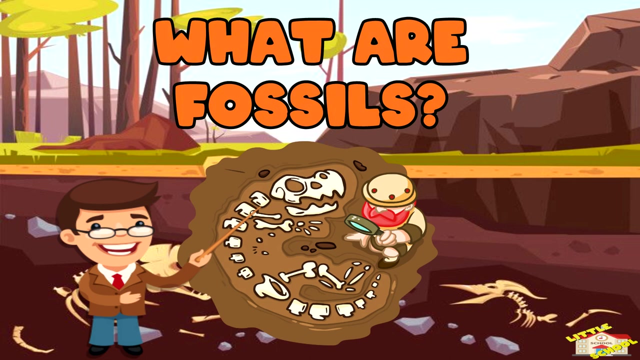 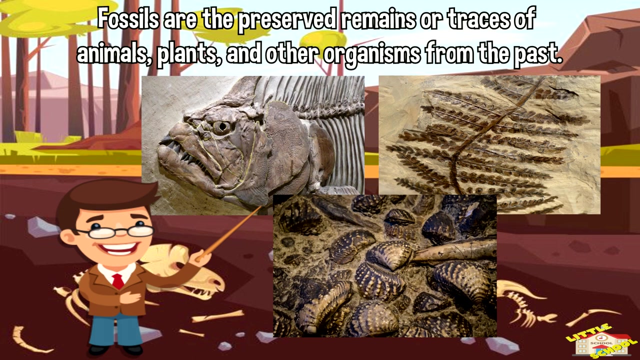 Hey kids, In today's video we'll be learning about fossils. Are you ready? Let's begin. What are fossils? Fossils are the preserved remains or traces of animals, plants and other organisms from the past. Fossils can be bones. 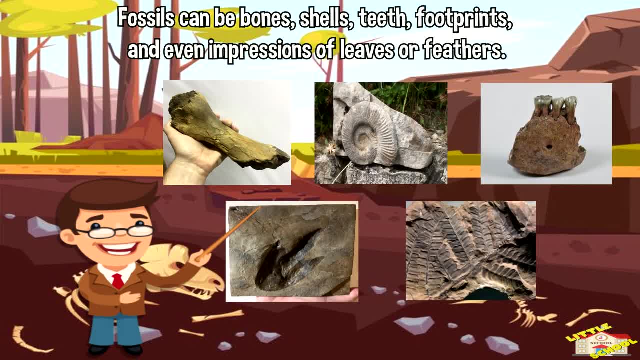 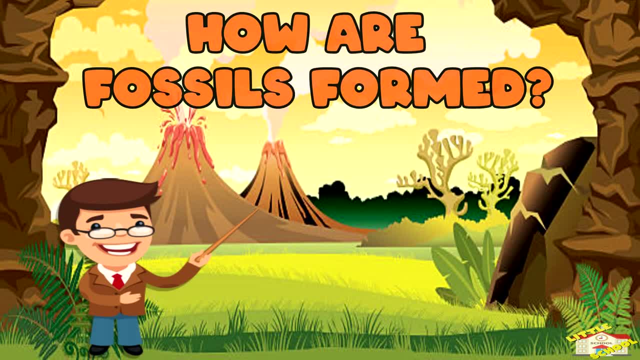 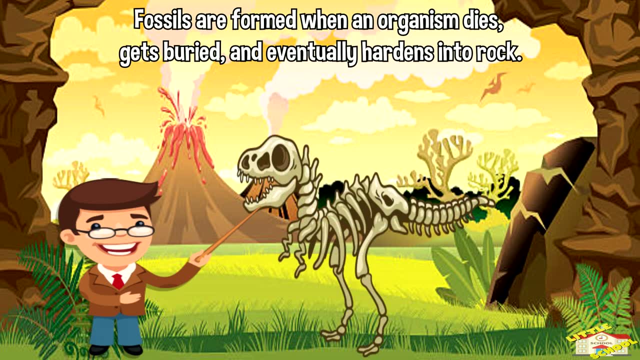 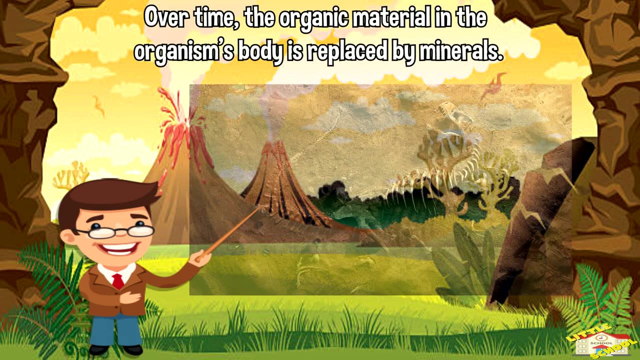 shells, teeth, footprints and even impressions of leaves or feathers. How are fossils formed? Fossils are formed when an organism dies and its remains are buried in sediment like mud or sand that eventually hardens into rock Over time. the organic material in the 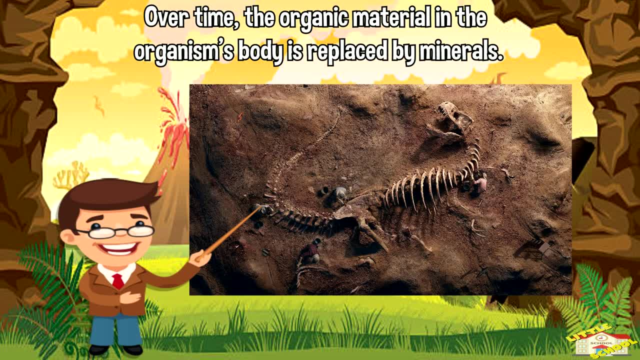 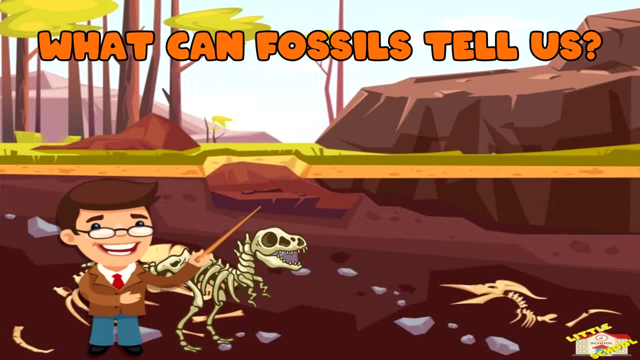 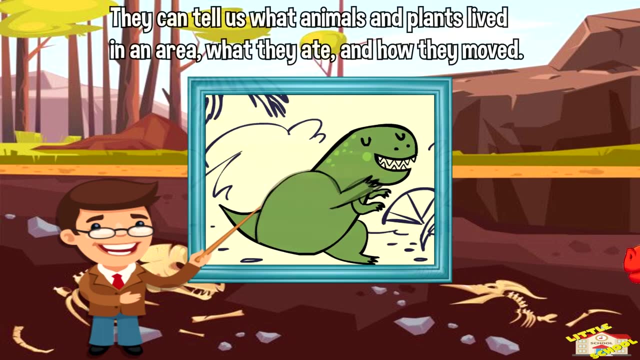 organism's body is replaced by minerals, leaving behind a rock-like copy of the original organism. What can fossils tell us? Fossils can tell us a lot about what life was like in the past. They can tell us what animals and plants lived in an area, what they ate and how they moved. 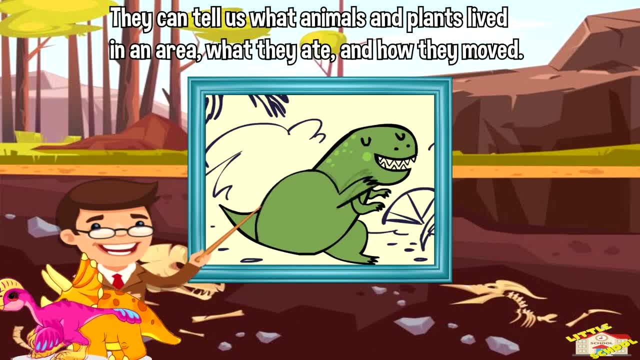 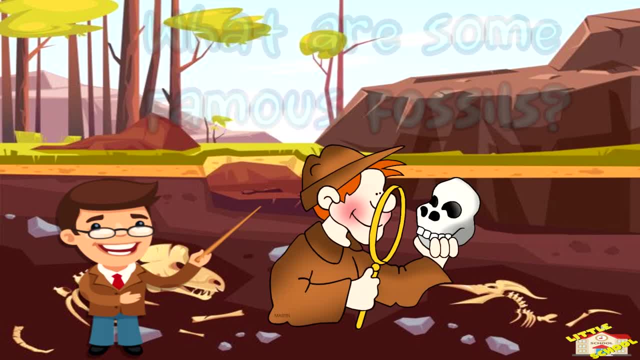 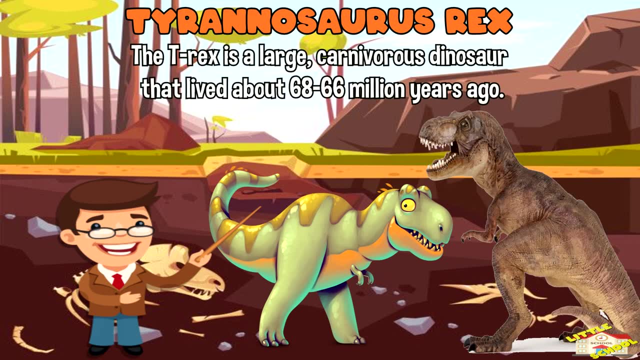 What are famous fossils? There are many famous fossils, but here are a few examples. Tyrannosaurus rex, The t-rex, is a large carnivorous dinosaur that lived about 68-66 million years ago. Many long seen faeces were useless when it was young, so it can be considered absolute. 이�وقing. 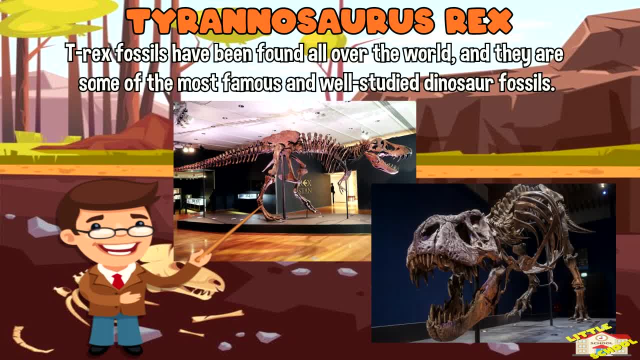 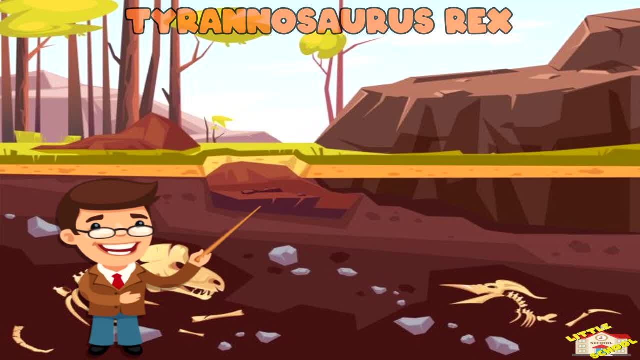 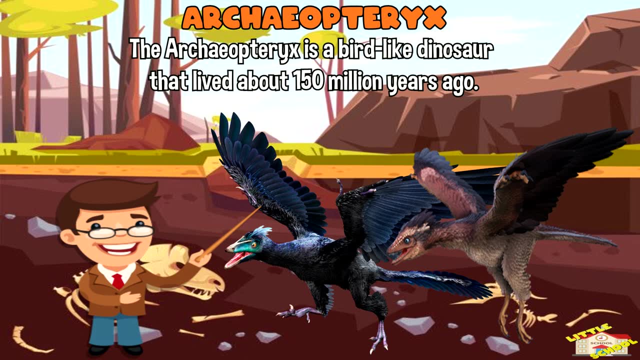 T rex fossils have been all over the world and they are some of the most famous and well studied dinosaur fossils: The Archaopteryx. The Archaopteryx is a bird-like dinosaur that lived about 150 million years ago. 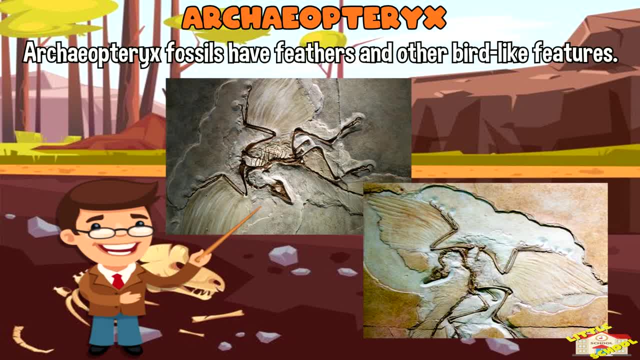 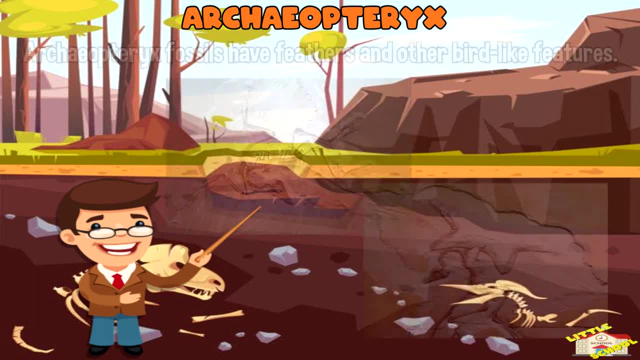 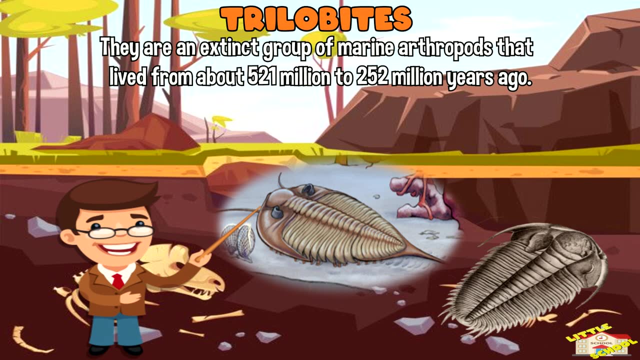 Archaopteryx fossils have feathers and other bird-like features, but also have teeth and a long bony tail, which makes them a transitional fossil between dinosaurs and birds. Trilobites: They are an extinct group of marine arthropods that lived from about 521 million to 252 million. 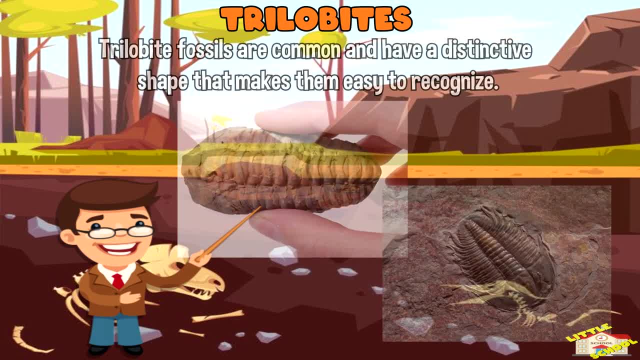 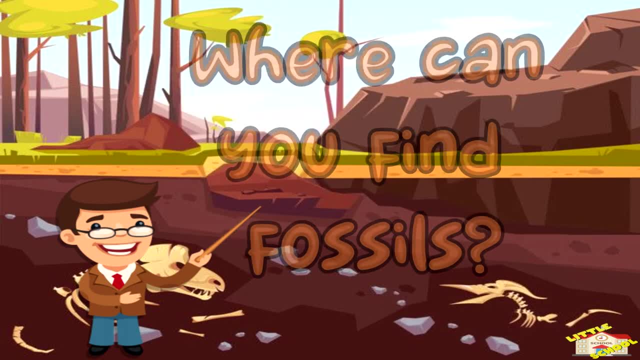 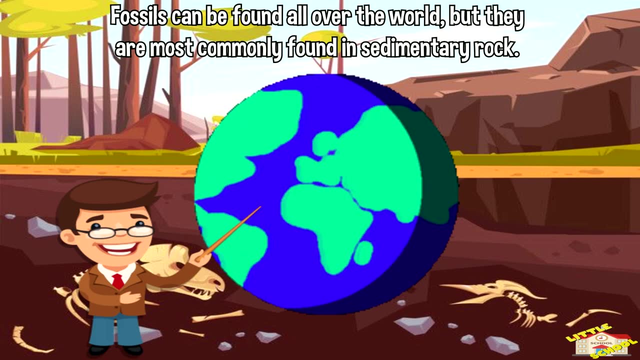 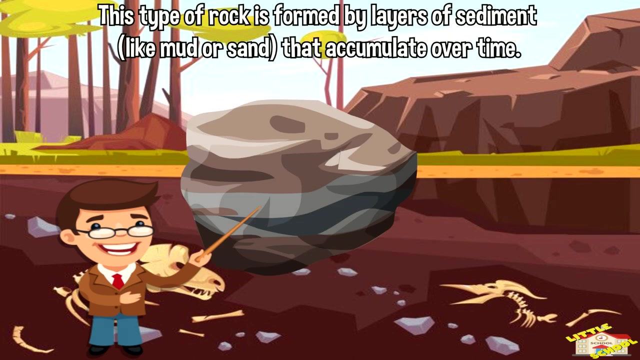 years ago. Trilobite fossils are common and have a distinctive shape that make them easy to recognize. Where can you find fossils? Fossils can be found all over the world, but they are most commonly found in sedimentary rock. This type of rock is formed by layers of sediment, like mud or sand, that accumulate over time. 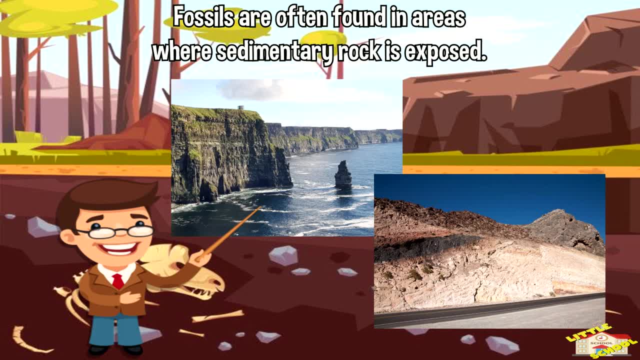 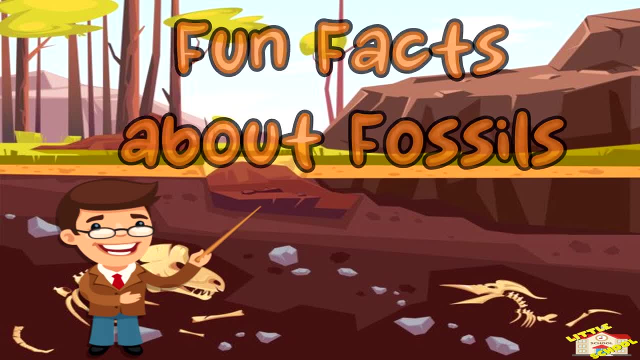 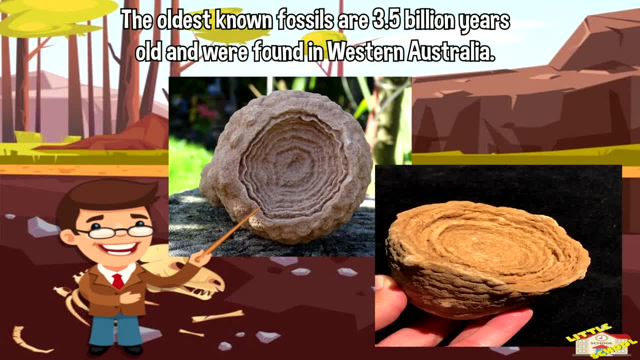 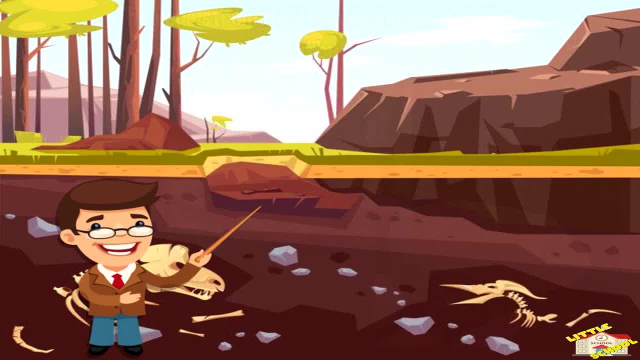 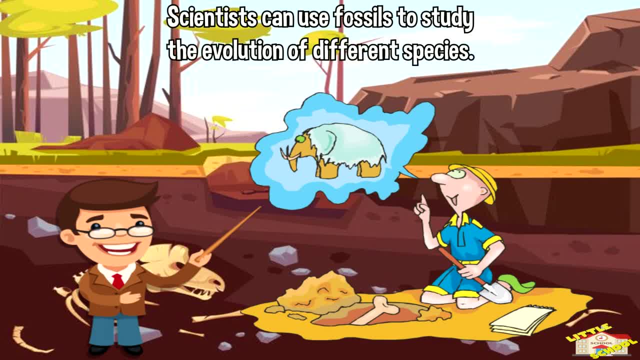 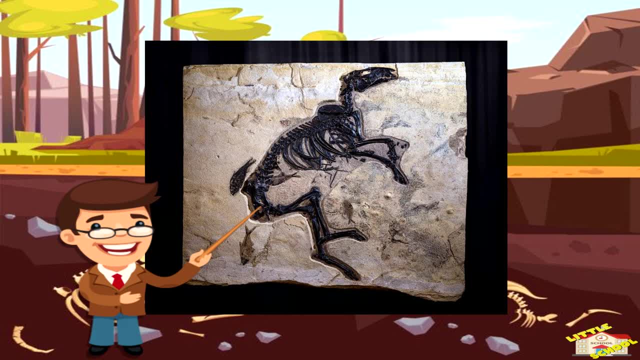 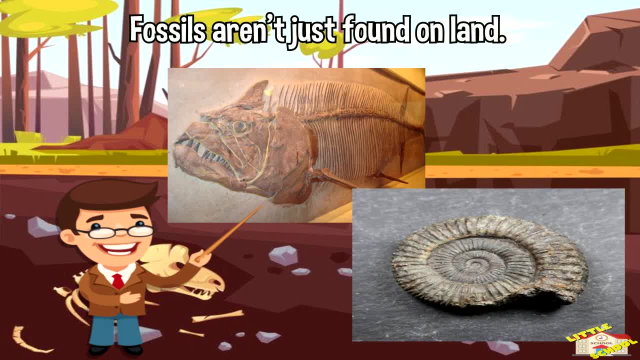 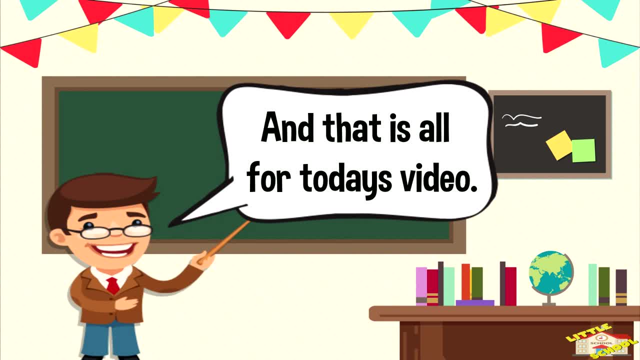 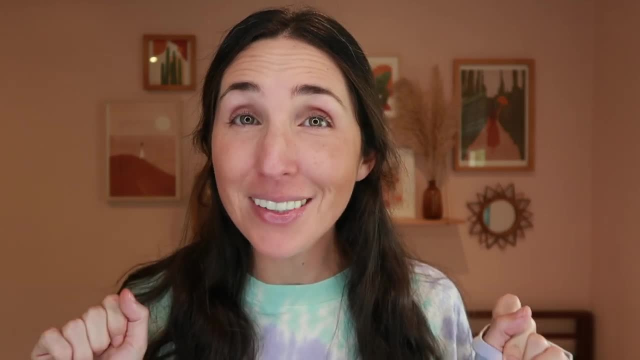 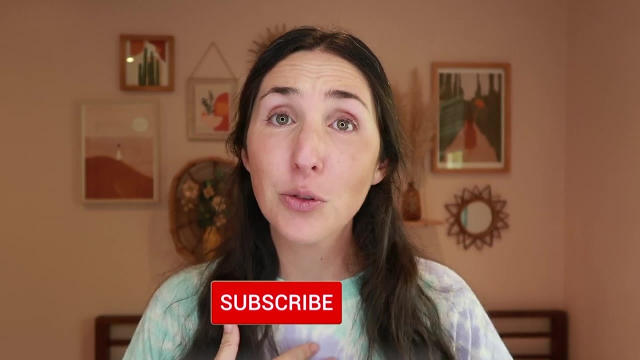 Looking to make easy, soft edible playdough in minutes. Today I'm sharing my go-to recipe: literally the best. It feels just like the real thing. If you guys are new here, my name is Rachel from The Confused Millennial. I share tons of kids activities, mom story at home tips and more I.